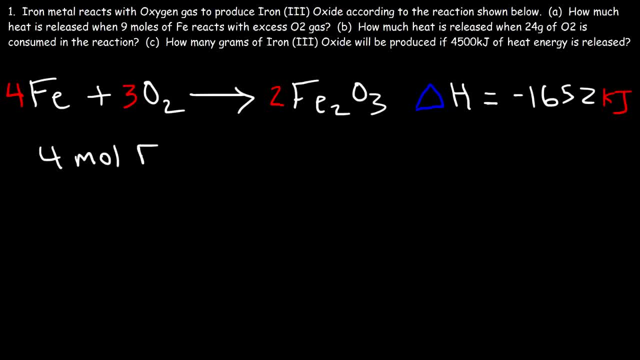 example, if four moles of iron metal reacts in this reaction, negative, sixteen fifty-two kilojoules of heat energy will be released. If three moles of oxygen gas is consumed in this reaction, the same amount of heat energy will be released. And if two moles of iron oxide is produced in this reaction, 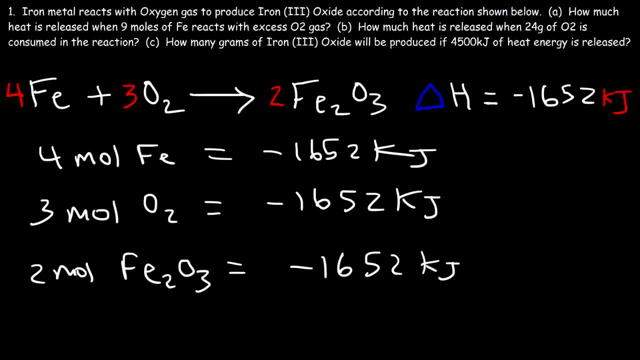 the same amount of carbon will be released. if the reaction is similar to the higher reaction amount of heat energy will be released. So you need to understand the relationship between this amount of thermal energy and the moles of the reactants and products. So now let's focus on this problem. 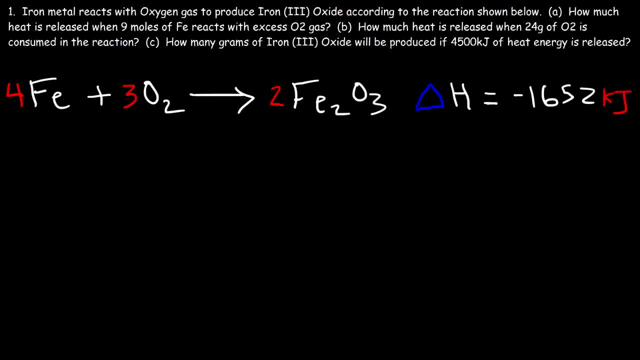 Iron metal reacts with oxygen gas to produce iron oxide, according to the reaction shown below, How much heat is released when 9 moles of Fe reacts with excess oxygen gas? So let's start with what we're given, and that's 9 moles of Fe. 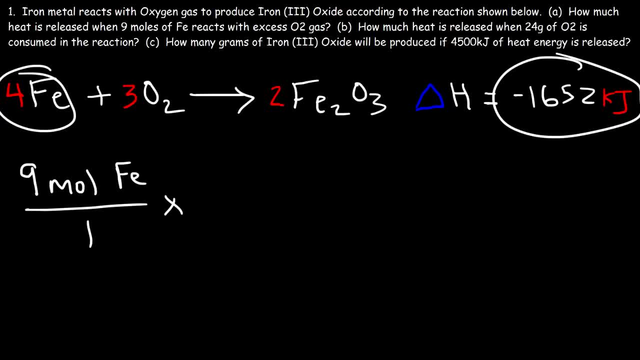 Our conversion factor is that 4 moles of Fe will generate 1652 kJ of heat energy. So we want the unit's moles of Fe to cancel. so we're going to put that in the bottom and put negative 1652 kJ on top. 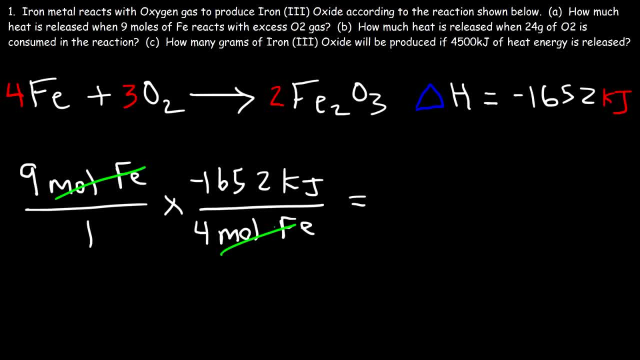 Okay, So these units will cancel, And so the answer is going to be 9 times 1652 divided by 4, 3717 kJ of thermal energy will be released if 9 moles of Fe reacts. So that's the answer to part A. Now let's move on to part B: How much heat is released? 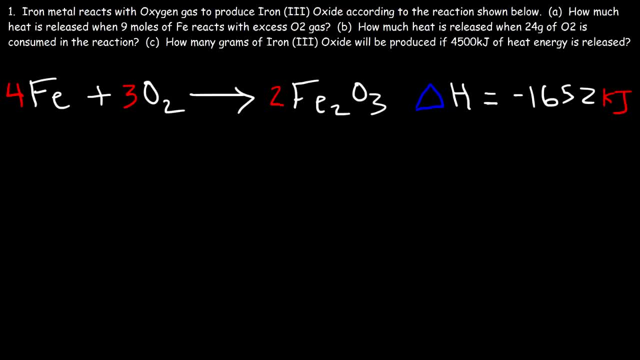 When 24 g of O2 is consumed in the reaction. Well, let's find out. So let's start with what we're given, that's 24 g of O2.. So if you're given a mass, what you need to do is you need to convert the grams to moles. 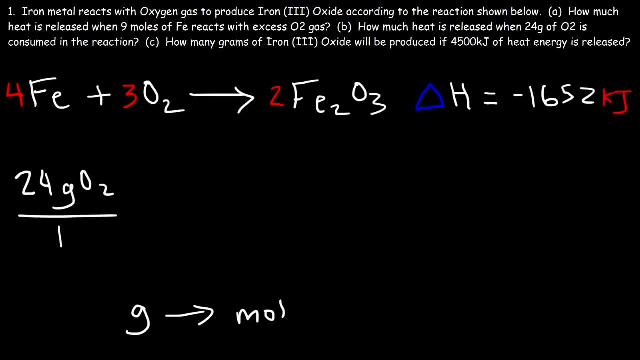 using the molar mass found in the periodic table, And then using the thermochemical equation, you can convert moles to kilojoules, And so that's what we need to do in this problem. So oxygen has an atomic mass of 16.. 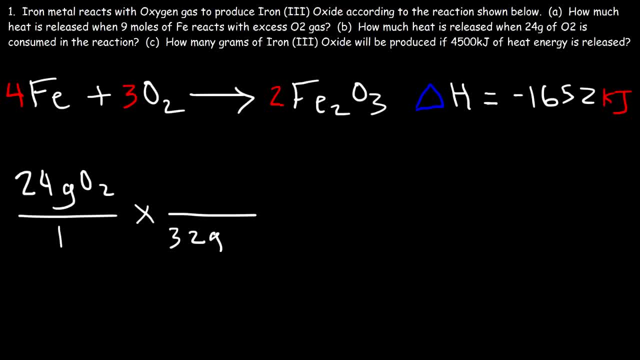 Therefore, O2 is going to be 16 times 2, which is 32 g per mole. So now that we have the moles of O2, we can use the fact that 3 moles of O2 would generate that amount of heat energy. 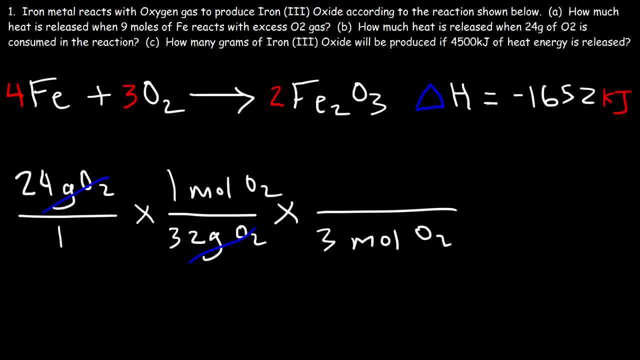 So I'm going to put 3 moles of O2 in the bottom so that the unit moles of O2 will cancel, And then 1652 kJ On the top of the fraction. So it's 24 divided by 32, which is 0.75 times 1652 divided by 3.. 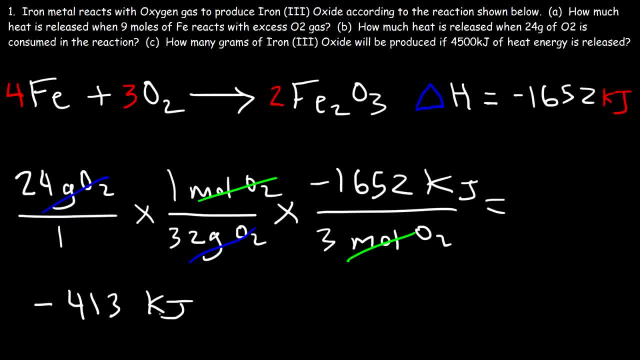 So it's negative 413 kJ of thermal energy. So that's how much heat will be released if 24 g of O2 reacts in this chemical reaction. Now let's move on to part C. How many grams of iron oxide will be produced if 4500 kJ of heat energy is released? 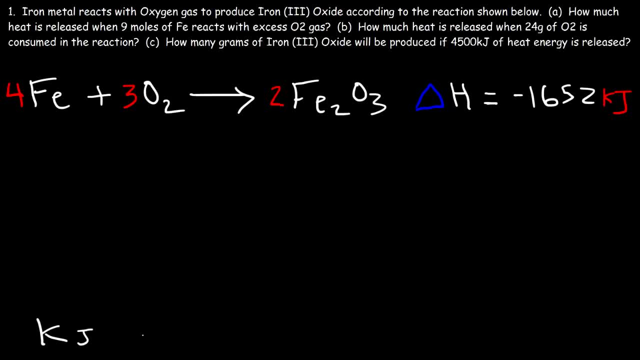 So this time we're given the amount of kilojoules. We need to convert it back to moles and then to grams. So let's start with what we're given, And that is 4500 kJ, And because this energy is released, it's negative. 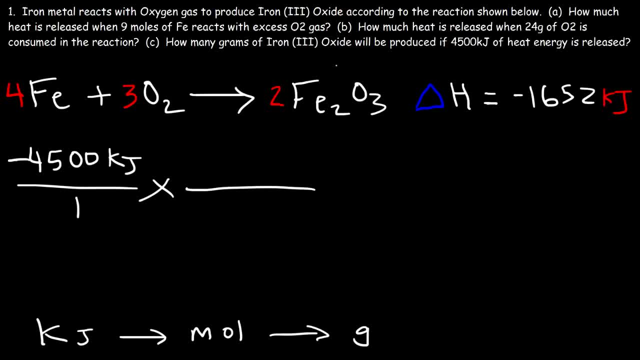 Now we can convert from kilojoules to moles using the fact that 2 moles of iron oxide corresponds to 1652 kJ. So negative 1652 kJ will be released when 2 moles of iron oxide are produced. 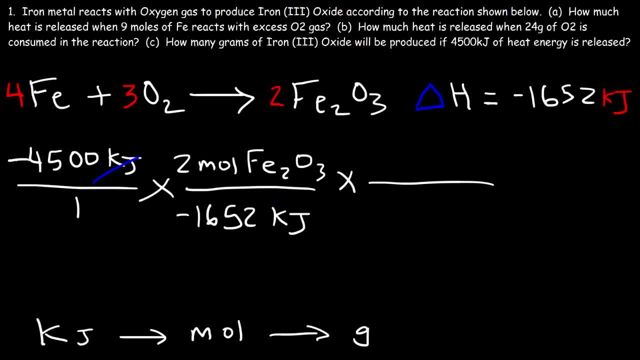 So now what we need to do is find the molar mass of Fe2O3.. So we have 2 Fe atoms and 3 oxygen atoms. So the atomic mass of iron is 55.85.. And for oxygen it's 16.. 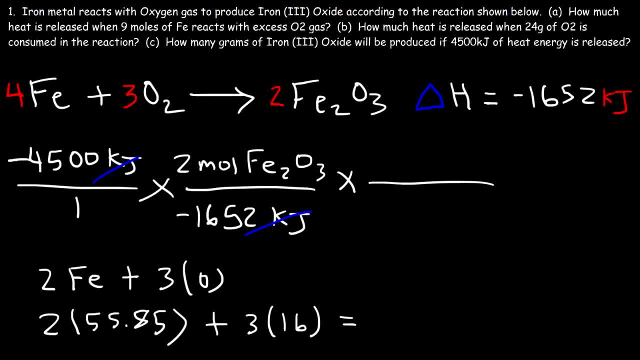 So the atomic mass of iron is 55.85.. And for oxygen it's 16.. So the atomic mass of iron is 55.85.. So ABCDE is 2 times 55.85, plus 3 times 16.. 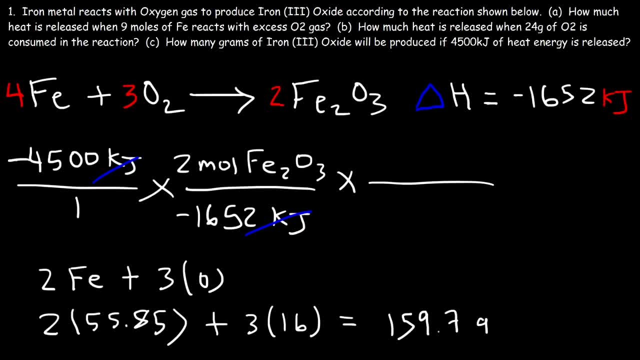 That will give us a molar mass of 159.7 grams per mole. So 1 mole of Fe2O3 has a mass of 159.7 grams. So now it's going to be 4500 times 2.2.. 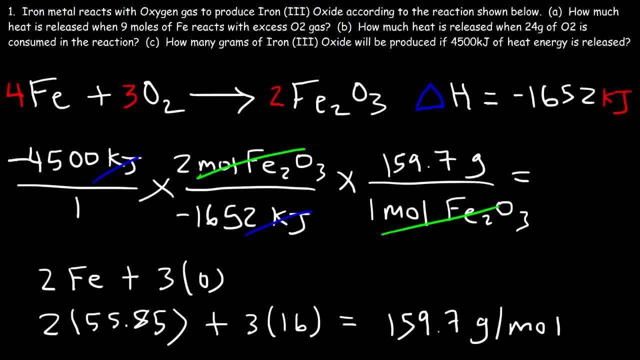 So what would that mean times 2, divided by 1652, and then take that result, multiply it by 159.7.. So the answer is about 870 grams of iron oxide. So make sure you know how to convert between grams and kilojoules when you're given a. 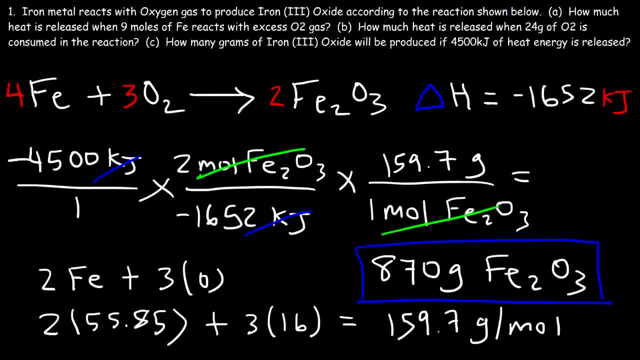 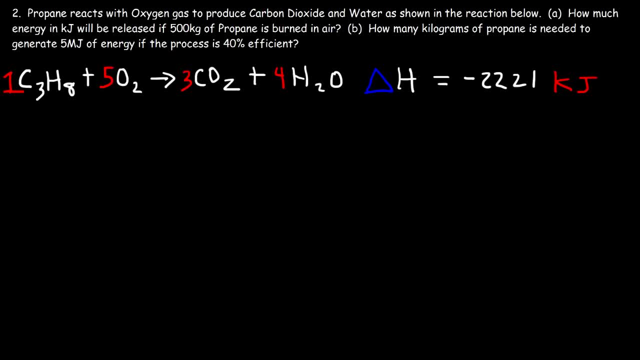 thermochemical problem like this one. Now let's move on to this problem. Propane reacts with oxygen gas to produce carbon dioxide and water. as shown in the reaction below, How much energy in kilojoules will be released if 500 kilograms of propane is burned in the? 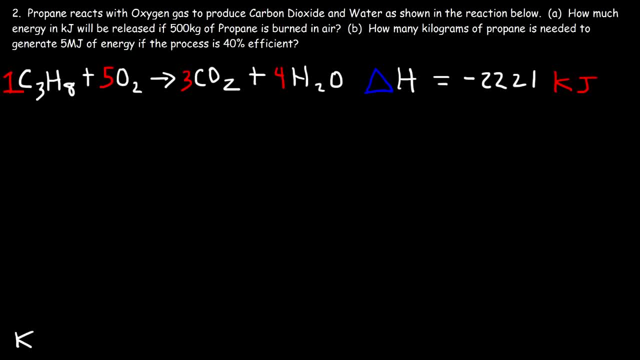 air. So we're given the kilograms of C3H8.. We need to convert it to grams and then use the molar mass to convert it to moles and then convert it to grams And then use the equation to convert it to kilojoules. 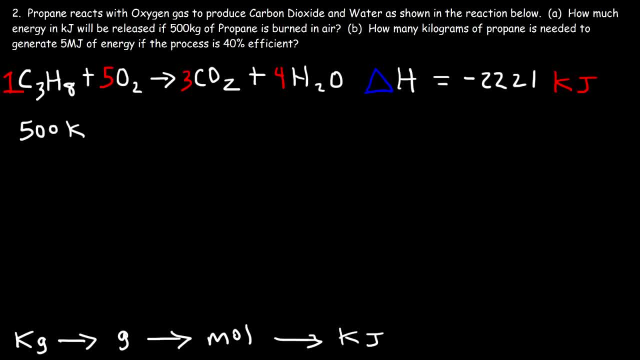 So let's start with 500 kilograms of propane. Now. 1 kilogram is equivalent to 1,000 grams And the molar mass of propane C3H8, it's going to be 3 times 12.0.. 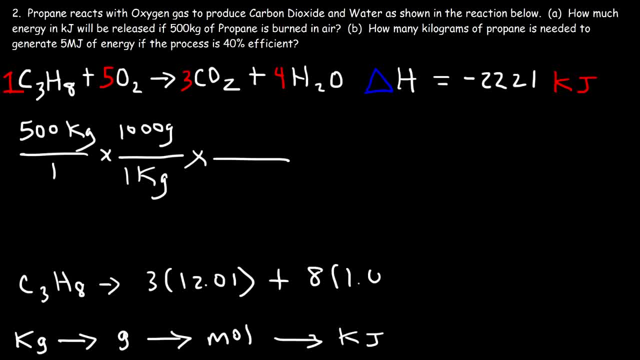 Plus 8 times 1.008.. So you should get this number. So I'm going to put one mole of propane on top and on the bottom 44.094 grams, And the substance is C3H8.. Now notice the ratio between C3H8 and the 2221 kilojoules. 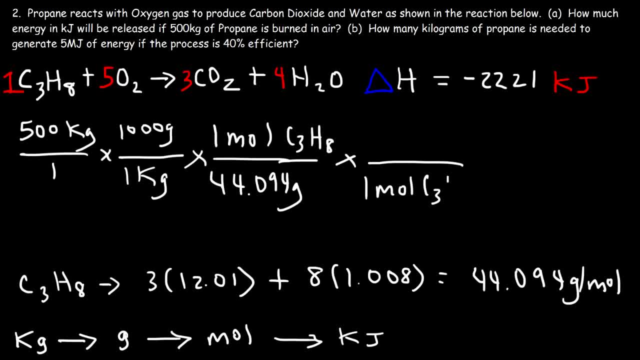 So the coefficient is 1. And 1 mole of propane will yield 2,221 kilojoules of heat energy. So now we're going to multiply 500 by 1,000, and then divide that by 44.094, and then multiply it by 2,221. 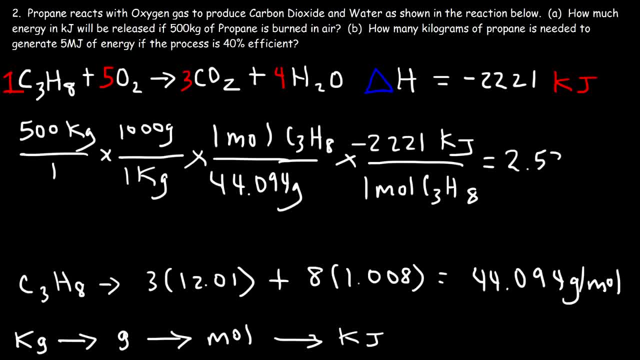 So you should get 2.52 times 10 to the 7th power kilojoules, And it's negative. So the exact answer is about 25,184,000.. That's 5,832 kilojoules. 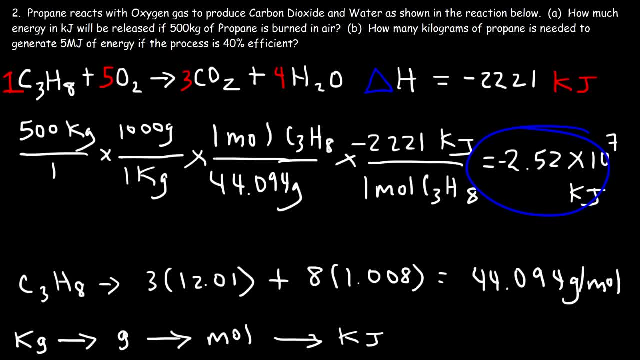 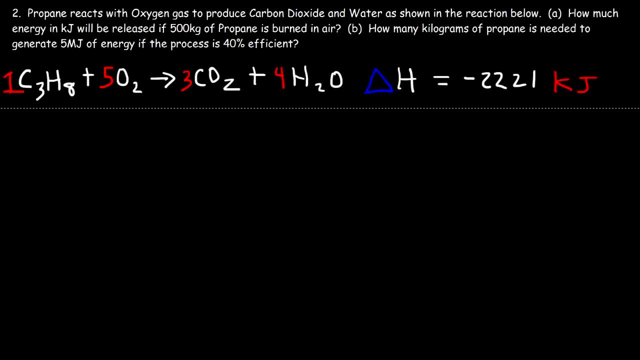 Now what about part B? How many kilograms of propane is need to generate 5 megajoules of energy if the process is 40% efficient. So we need to generate 500 megajoules of energy, And 40% of the energy that's released is going to generate 5 megajoules of energy. 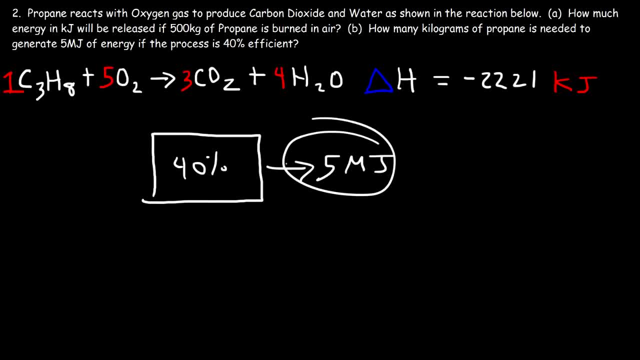 And 40% of the energy that's released will be in its usable form. The other 60% will be lost, maybe due to heat or something. It could be lost as friction, It could escape into the environment. But only 40% of the energy that's going to be released. that's the amount that we're going to capture and do something useful with it. 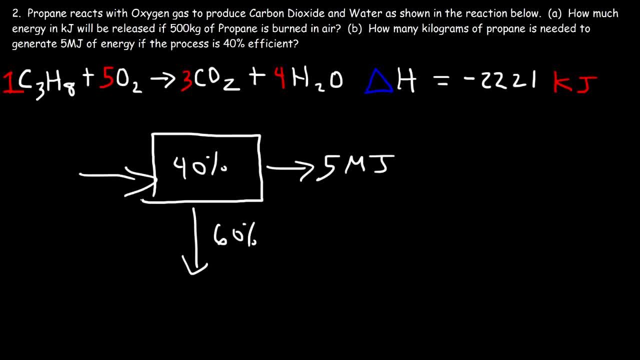 So how much do we need to begin with? So 40% of the energy that's going to be released is going to generate 5 megajoules of energy, And 40% of what number is 5?? To find that answer, you have to take 5 and divide it by 40%. So 5 divided by 0.4 is 12.5.. So we need to determine the amount of propane that we need to burn to generate 12.5 megajoules of heat. Once we generate that amount of heat, we can capture 40% of it, which represents 5 megajoules. 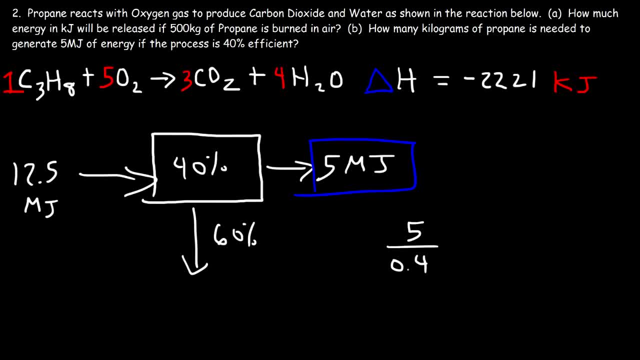 The other 60%, which is 12.5 times 0.6, that's going to be lost to the environment, So that's going to be waste energy. So we need to convert this value to kilograms of propane. So let's start with 12.5 megajoules of energy. 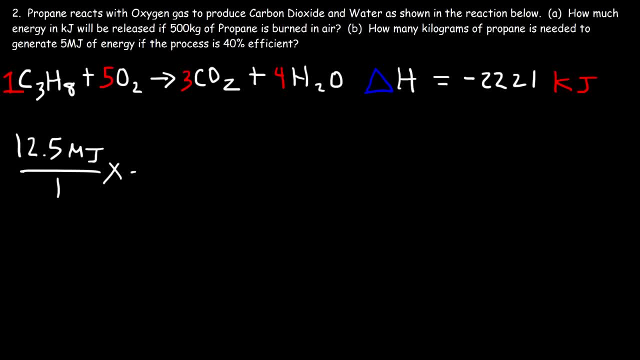 Now, before we do that, let's look at the value of propane. Before we can use this number, we need to convert megajoules into kilojoules. One megajoule is equivalent to 1,000 kilojoules. 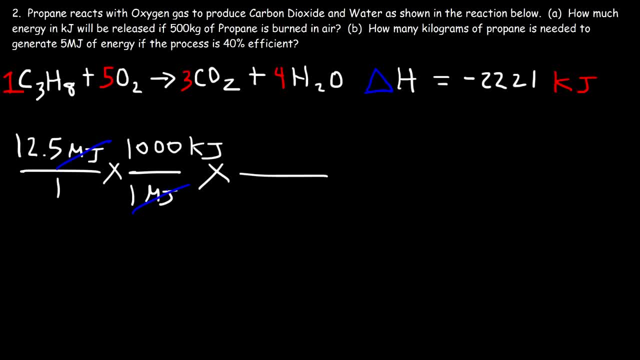 So now that we have the energy in kilojoules, we can convert it to the moles of propane. So for every 2,221 kilojoules that we have, one mole of propane needs to be consumed. So now let's convert moles of propane into grams. 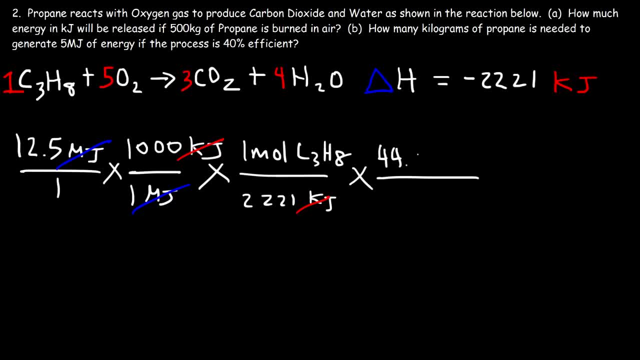 So the molar mass was 44.094 grams per 1 mole of propane. Now the last thing we need to do is convert grams to kilograms. So there's 1,000 grams per kilogram, And so that's it for the conversion. 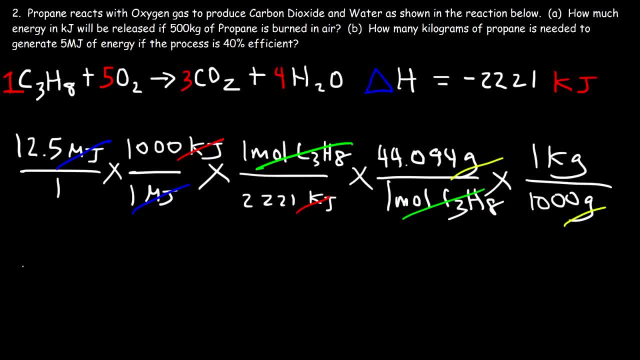 So now all we got to do is just plug in the values that we have. So it's going to be 12.5 times 1,000 divided by 2,221, multiplied by 44.094 divided by 1,000.. 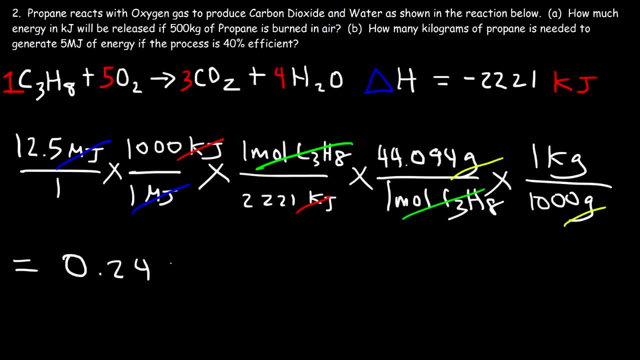 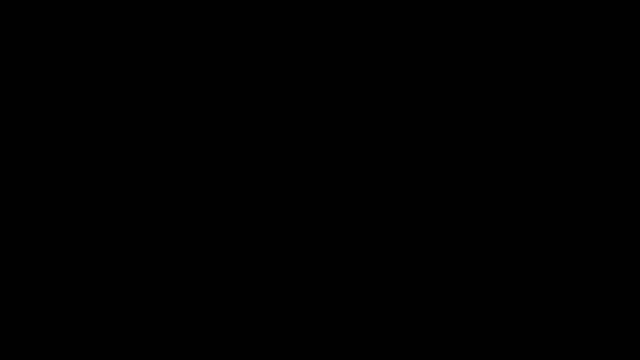 So this is going to be 0.248 kilograms, So that's how much kilograms of propane that we need to burn in order to generate 5 megajoules of energy if the process is 40% efficient. Thank you,